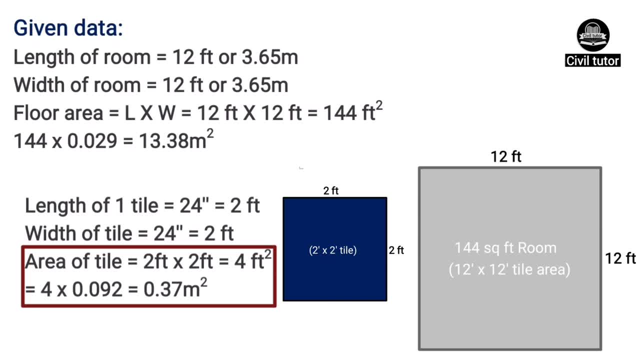 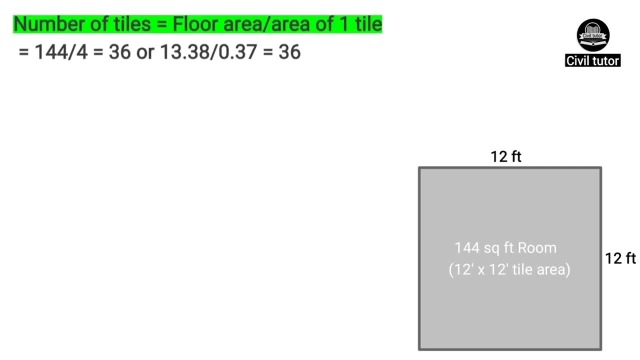 So the area will be 2 feet x 2 feet, which will be equal to 4 square feet, or simply 0.37 meter square. The number of tiles will be calculated by using the formula floor area upon area of one tile. Floor area is equal to 144 square feet and area of one tile equal to 4 square feet. 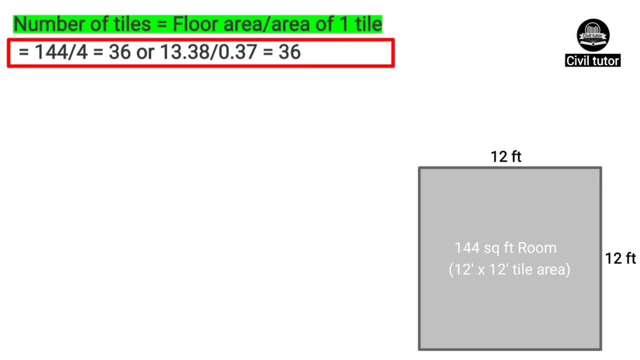 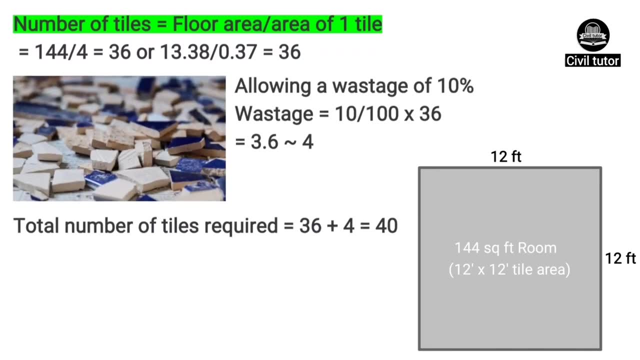 So, on substituting these values, we will get the number of tiles equal to 36.. Now allowing a wastage of 10%, that is, 10% of 36, which is equal to 4.. Hence, the total number of tiles required will be equal to 36 plus 4, which will be equal to 40.. 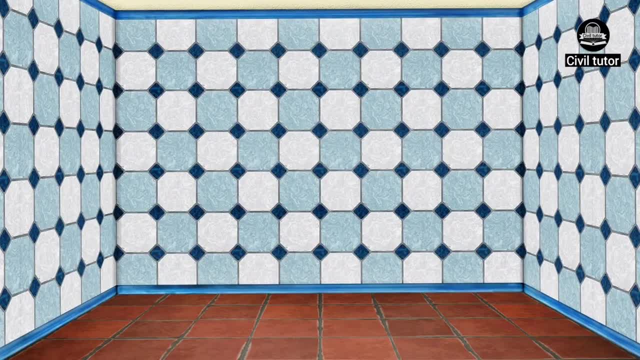 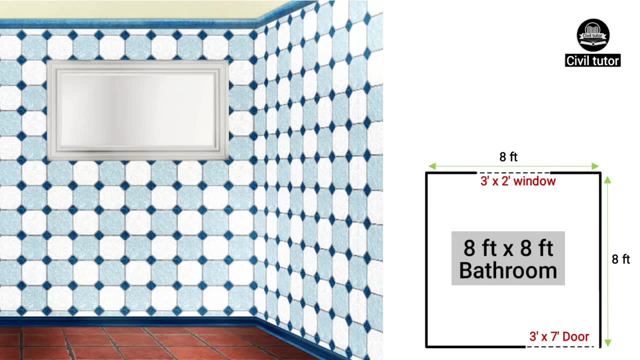 To calculate the number of tiles required for a wall area. let's quote another example to make it easy for you. Suppose we have a bathroom of size 8 feet x 8 feet, the height of its walls is 9 feet and we need to calculate the wall tiles. 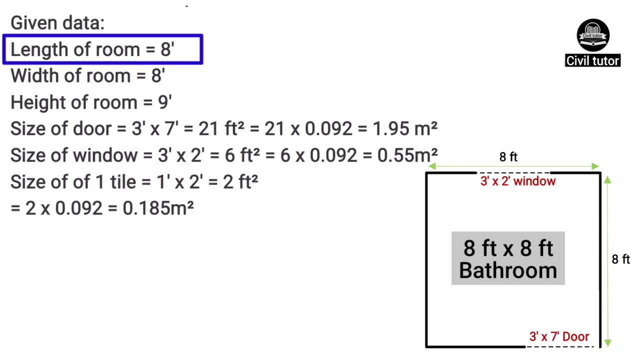 So we have the given data: Length of room is 8 feet and width of room is also 8 feet. The height of room is 9 feet. Size of door is 3 feet x 7 feet, which will be equal to 21 square feet. 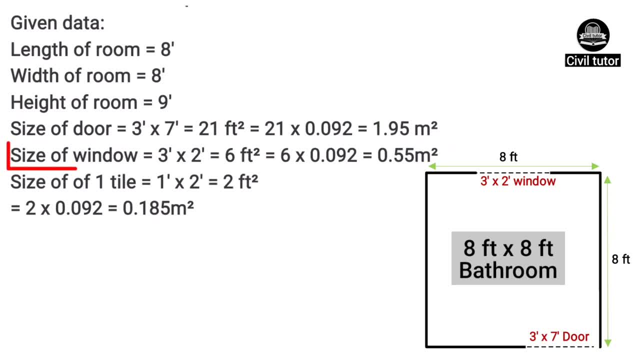 or 1.95 meter square. The size of window is 3 feet x 2 feet, which is equal to 6 square feet or simply 0.55 meter square. The size of one tile is taken as 1 feet x 2 feet, which is equal to 2 square feet or 0.185 meter square. 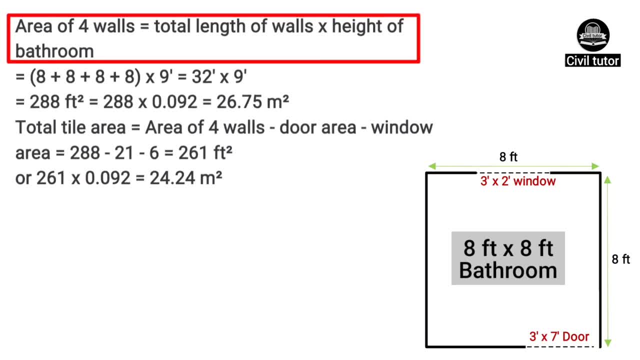 The area of four walls will be equal to total length of walls, into height of bathroom, which will be equal to 4 times 8, into 9, equal to 285 meter square. This will be equal to 288 square feet, or simply 26.75 meter square. 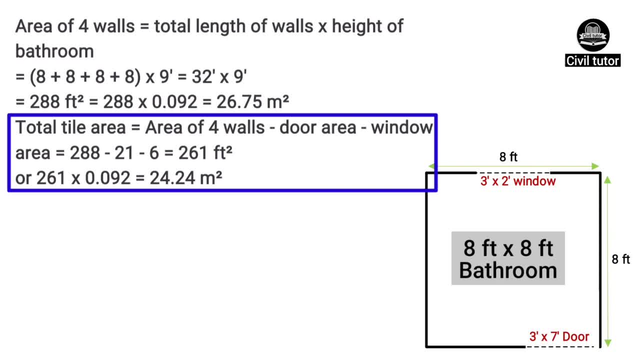 Total tile area will be equal to area of four walls minus door area, minus window area, which will be equal to 288 minus 21 minus 6, equal to 261 square feet or 24.24 meter square. Number of tiles will be calculated by using the formula.